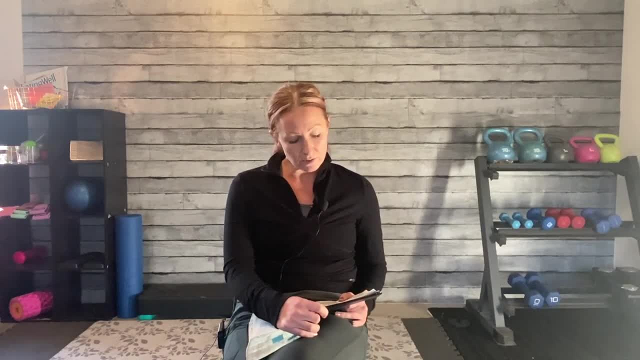 see, I have given you a gift of life. I have given you a gift of life. I have given you a gift of life. I have given you every herb that yields seed which is on the face of all the earth, and every tree whose fruit yields, yields seed to you. It shall be for food also to every beast of. 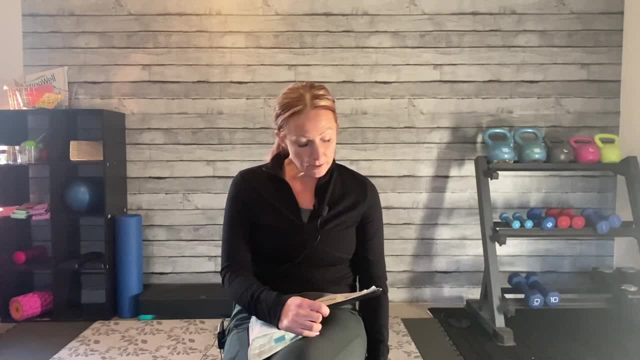 the earth, to every bird of the air and to everything that creeps on the earth in which there is life. I have given every green herb for food, And it was so so here in the beginning, when God created us cause. we know we're. 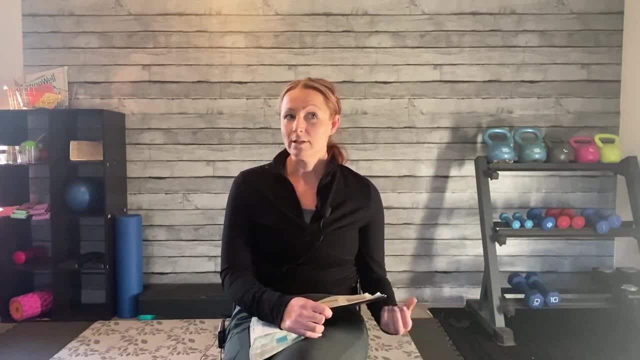 God's creation. He created our food. We're a living being. He created all the animals, And he also gave us the food that is to nourish our bodies, And so, to me, what stuck out is everything that creeps on the earth in which there is life, And we're a living being. 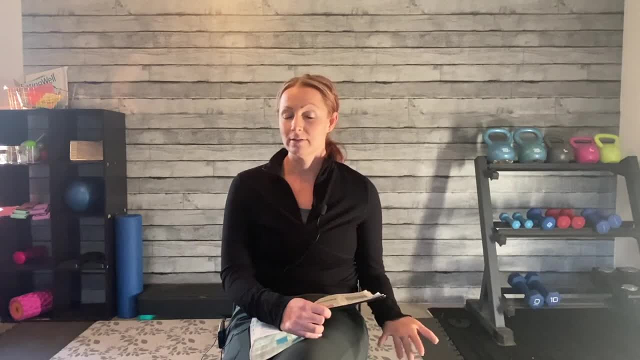 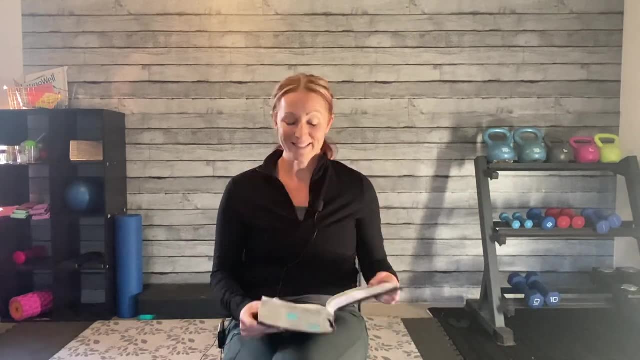 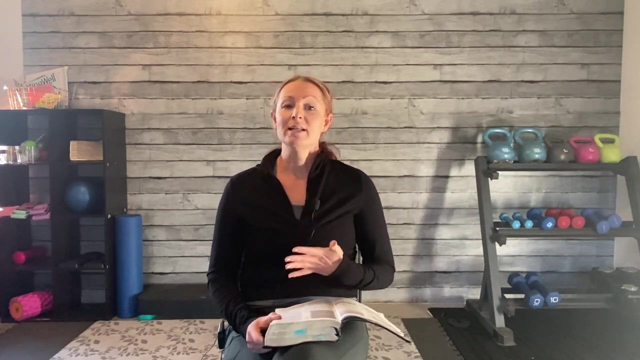 which means we need living food. That's really what it comes down to. We read a Bible- Hopefully, all of us do- And the scriptures say that the word is living and powerful and sharper than any two edged sword. So I know and I have experienced that this Bible comes alive. 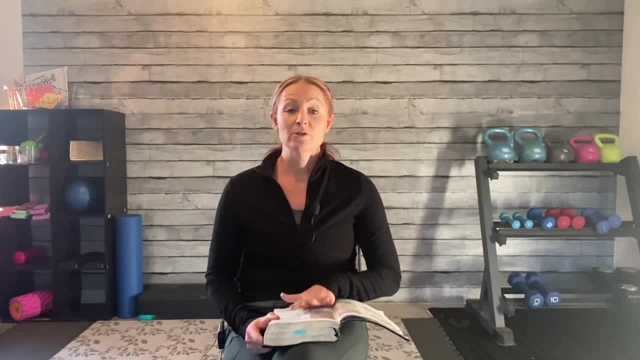 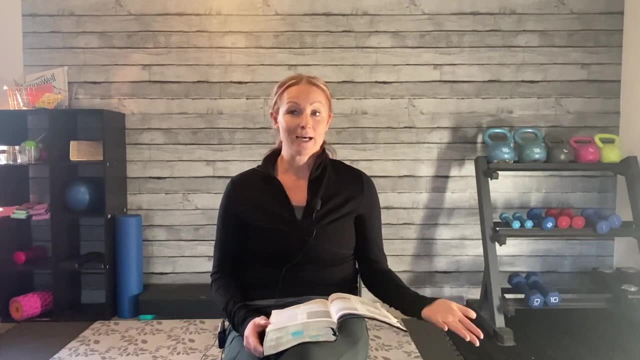 It applies to me every day And I can read these scriptures every day because it's living. We also serve a living God. If we didn't serve a living God, why are we serving Jesus? He's alive. He rose from the grave. 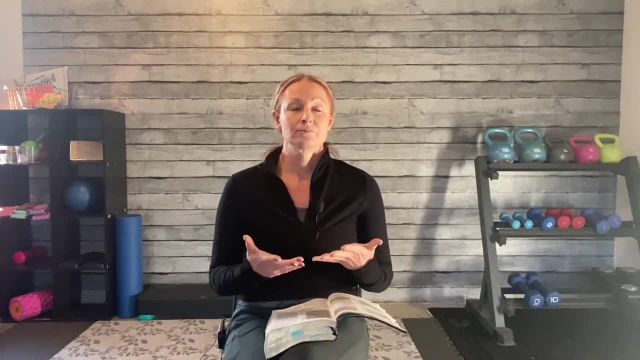 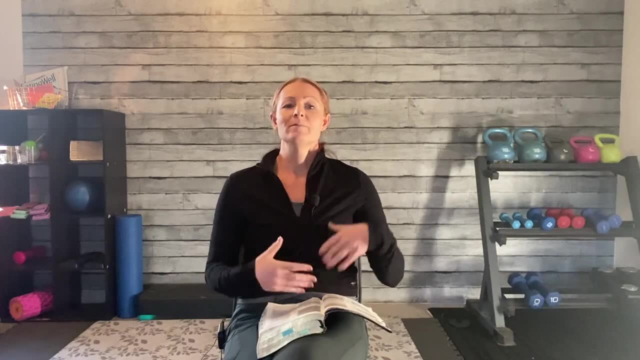 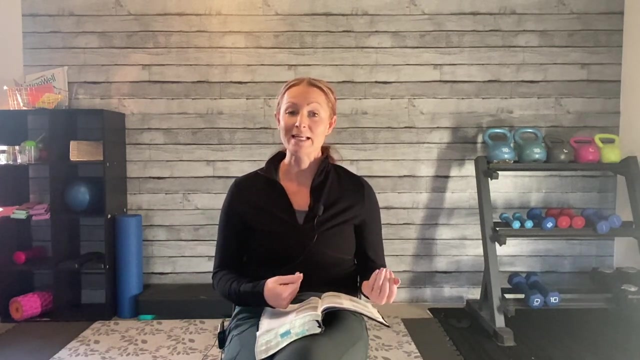 He's living. So to me, that word living really touched me because if we are a living being, we need our spiritual food from a living God And if the natural proceeds the spiritual, we also need living food to nourish our bodies, And from the beginning of time. 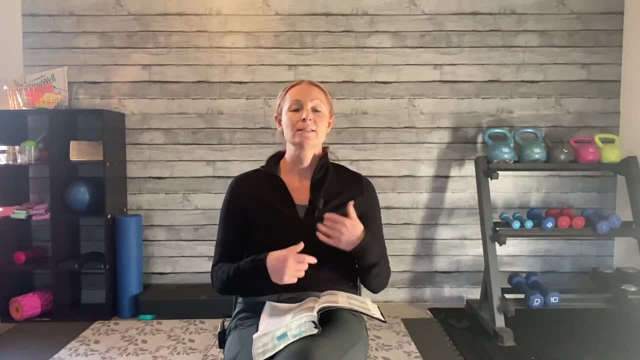 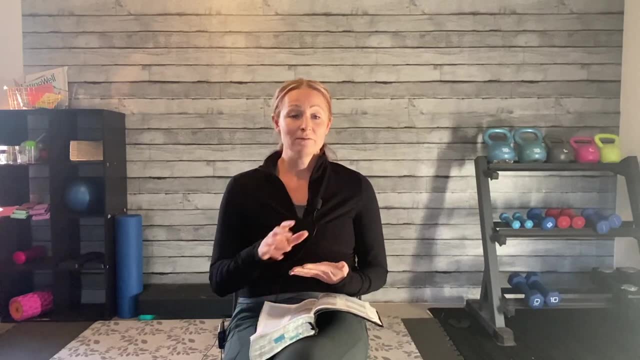 God has already created the food that will heal our bodies, to nourish our bodies And, in the scheme of things, you know the world, man-made food, the chemicals in our food. we eat so much dead food and then we expect to be. 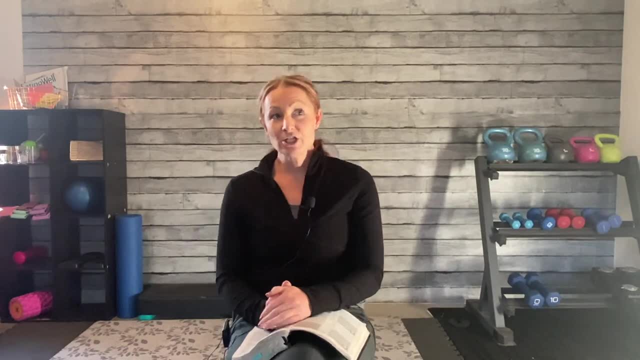 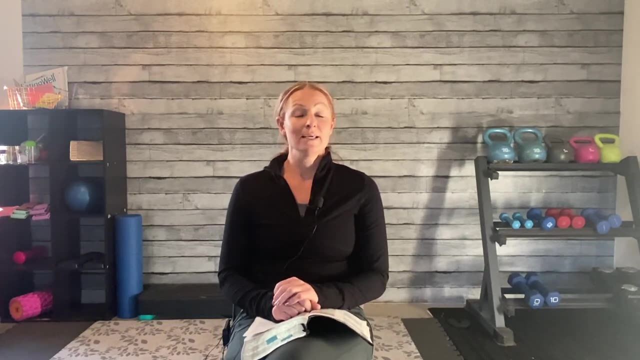 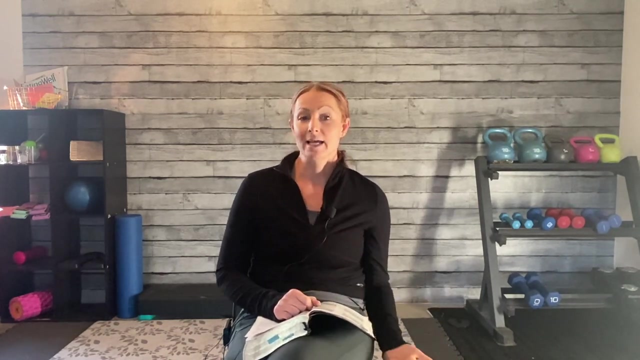 nourished and to be healed. So when I had changed my diet to adding a lot more living foods- green juices, which are full of enzymes- into my diet, I really saw drastic changes. So I really believe in the power of the food God created And for me that is eating a lot of. 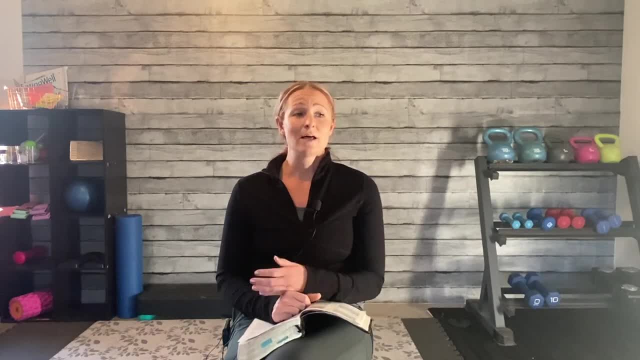 fruits and vegetables, And for some people it's eating a lot of fruits and vegetables, And for some people it's eating a lot of vegetables, And for some people it's eating a lot of fruits and vegetables, And for some people that is just adding in a lot of green juice to your diet to get. 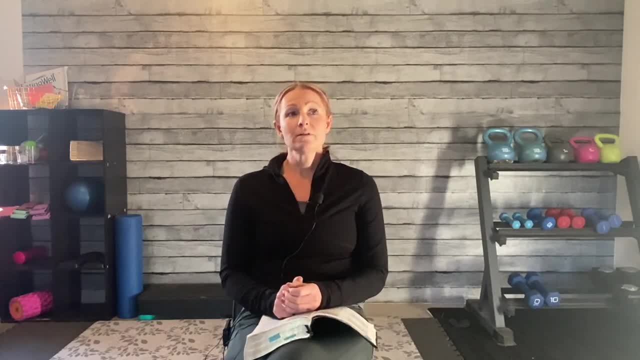 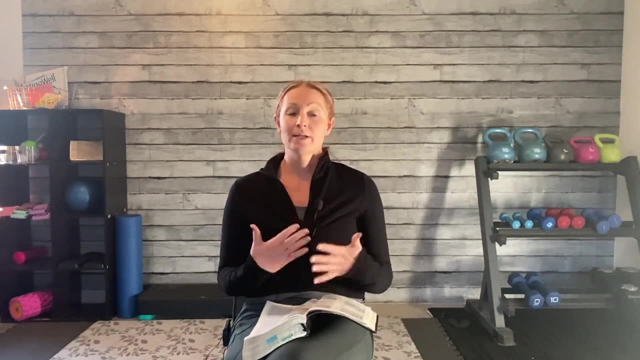 the enzymes that your body needs. So for those of you who don't know what enzymes are, it's quite literally the building block of your body. Everything in your body, every cell of your body requires enzymes, And without enzymes we actually wouldn't be able to function. 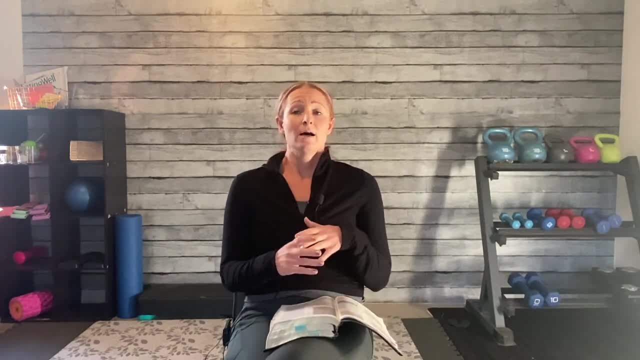 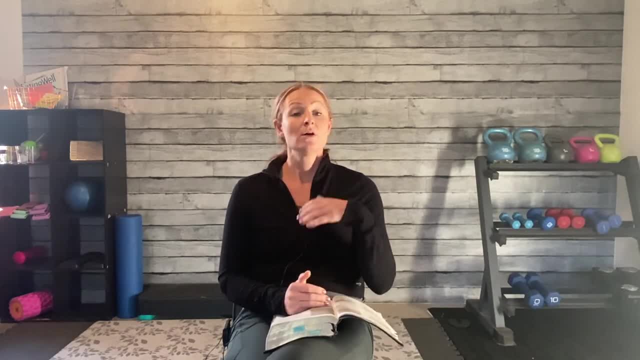 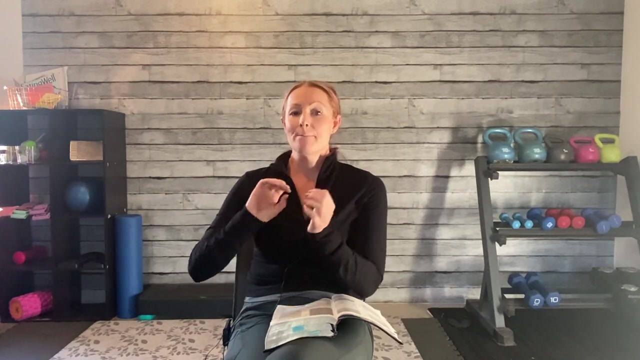 So how the living food works is: you're getting the enzymes from the vegetables, from the fruit, from the green juice. The green juice is really a way to break down and separate the fiber from all the vitamins, the minerals and the enzymes. So I would encourage you guys to. 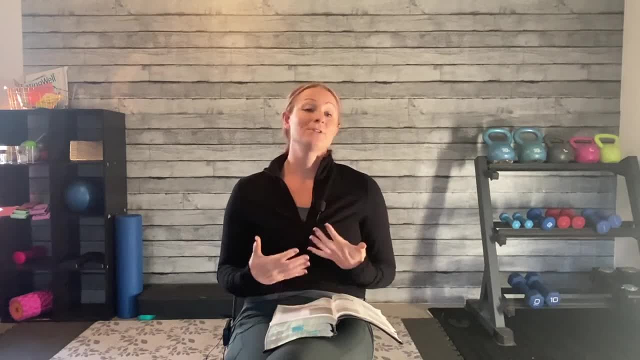 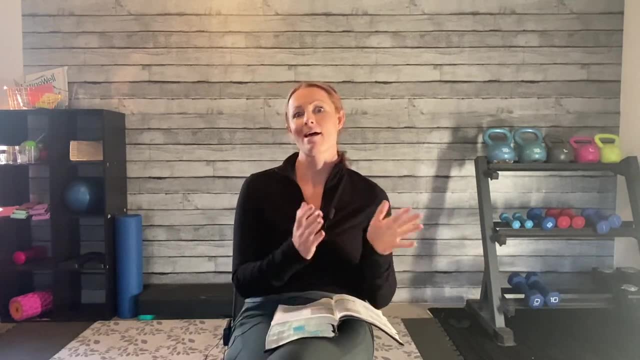 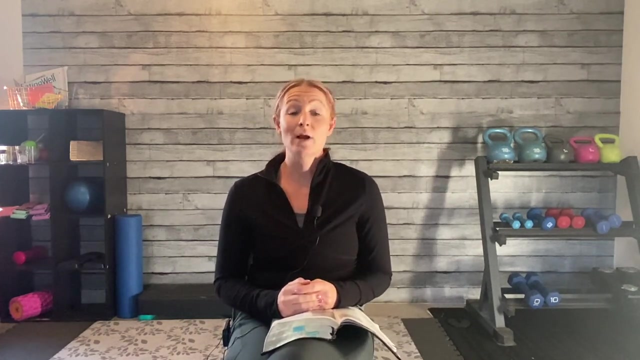 if you don't already, to try to add in as much fruits and vegetables that you can Add in a green juice to your salad or your eggs for breakfast or wherever you can get in the vegetables. I would just recommend trying it, seeing how you feel. We know, guys, that we're in a war right now. 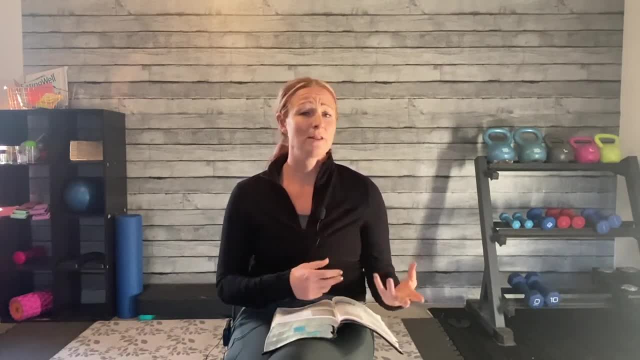 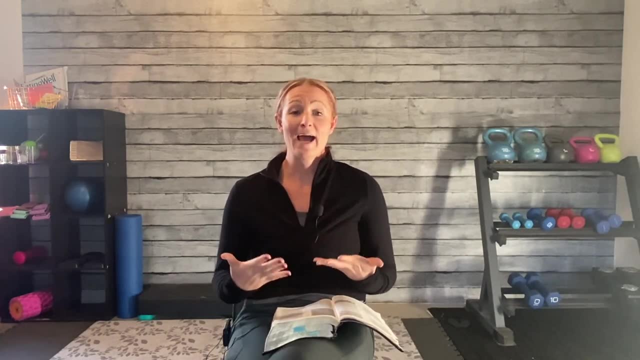 You know, COVID-19 is everywhere. There's health everywhere, There's sickness everywhere And we're in a battle And the battle that we have, we have our bodies as our weapon. It's our strongest weapon that we have. If you're going to go into battle with your gun, you know. 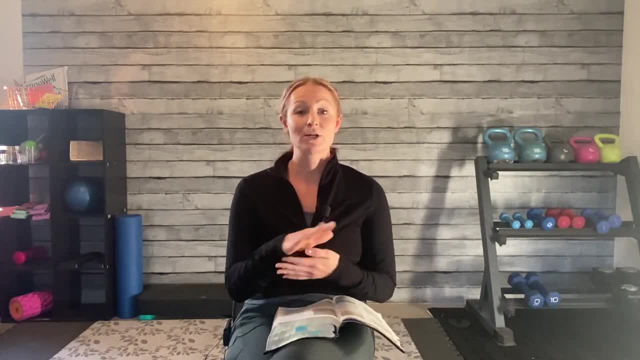 you're going to clean your gun before you go. I don't know any officer or anybody who's going to go shooting and they do not check their gun. They clean their gun to make sure that when you're going to go pull the trigger it actually works, Because if you don't keep your gun clean, 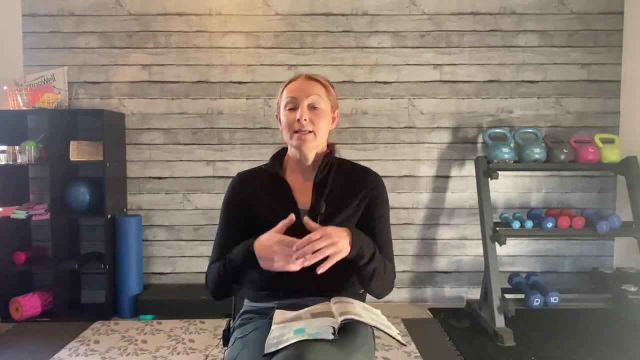 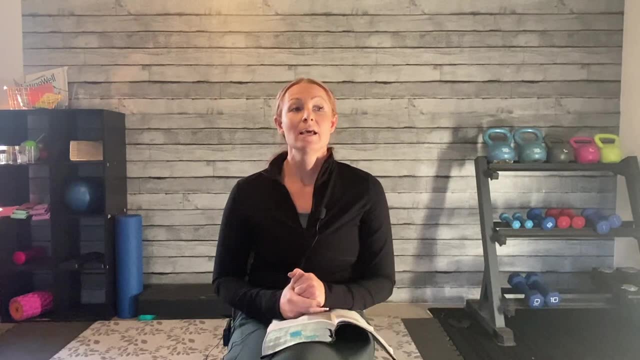 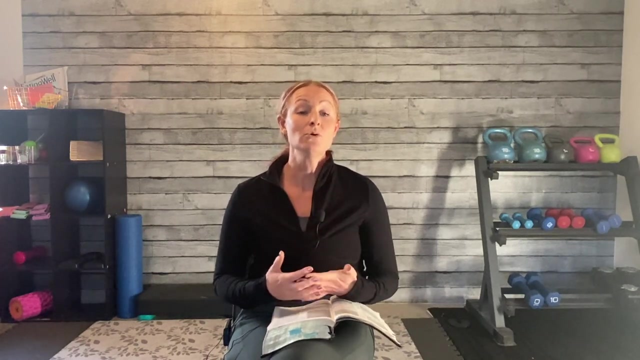 it's not going to work. So, to me, my body is a weapon. It's a weapon to fight against disease, to fight against these illnesses that come to us. And so you know, the scriptures tell us that our body is not our own. It's the temple of the Holy Spirit who is in you, whom you have from God, And 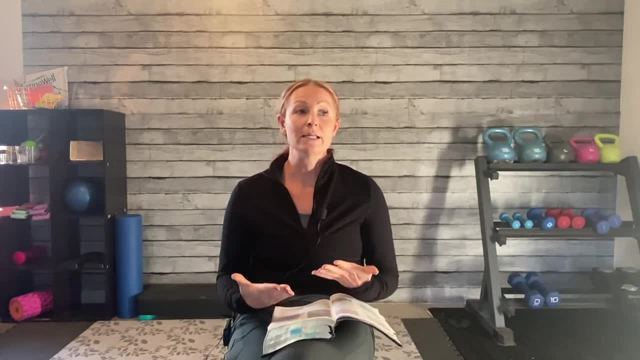 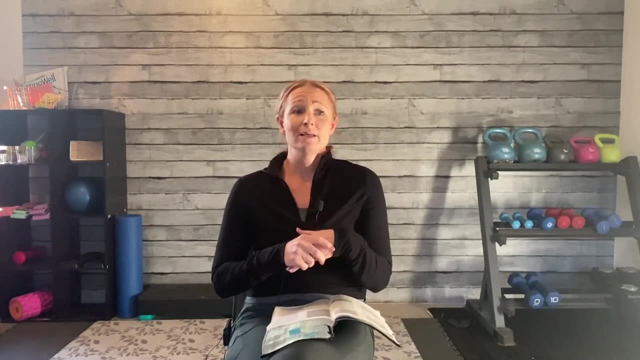 we're to honor our bodies with our soul and our spirit and to stay healthy. So it is almost a responsibility not to try to be lawful but to honor our bodies with our soul and our spirit and to stay healthy. So it is almost a responsibility not to try to be lawful. 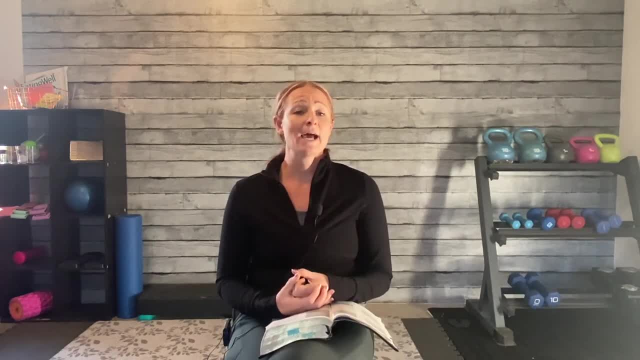 but to try to take care of our temple and to keep it healthy. so we have energy, we have endurance to stand our post, whatever that post is that God has called you to do. You know whether that's just raising your kids, or if you're preaching God's word, or if you're a fitness instructor. 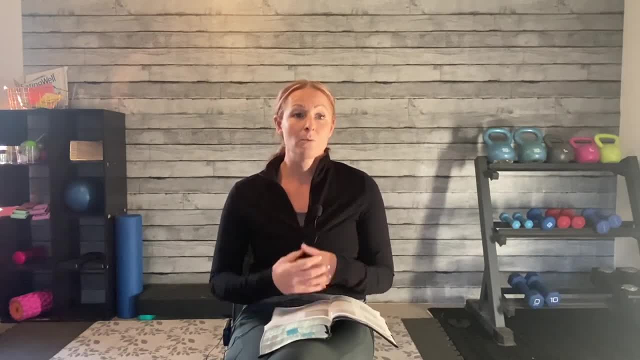 like Christina, if we don't have our health, we can't do any of those posts. So to stay healthy it's really important, guys, and it helps you just live a happier life. So I would encourage you guys to stay healthy. I would encourage you guys to stay healthy. I would encourage you guys. 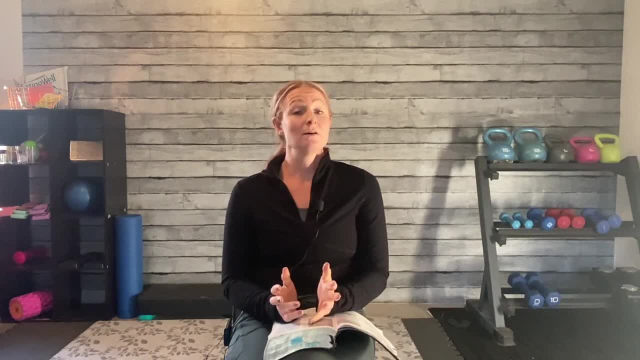 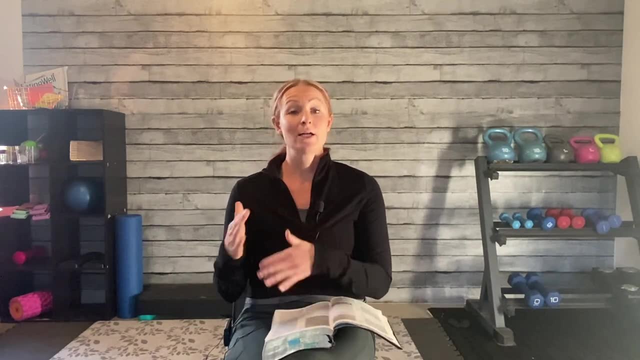 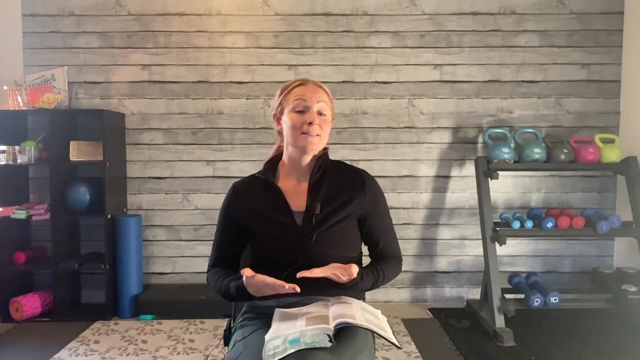 to just challenge yourself to take the sugar out, take some of these acidic foods out of your diet- maybe it's just one thing at a time- and try to replace it just little by little, with some of these foods that God created for us to eat. He created our bodies, guys. He is the most. 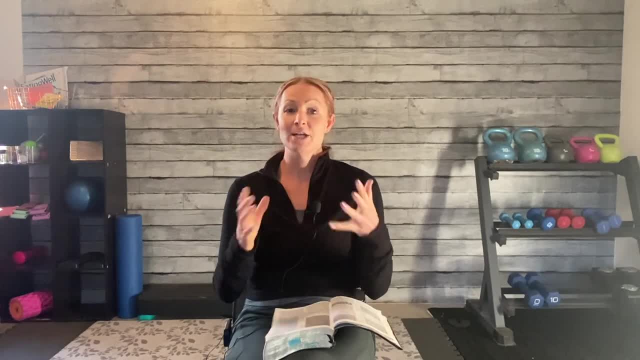 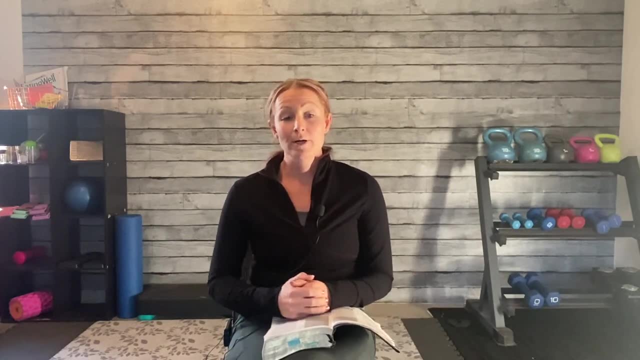 this body that we have is the most miraculous engine or machine that we have. Nothing can mimic what God created. So you know, if we have a car, we're not going to go put in the wrong oil, We're not going to go put in the wrong oil, We're not going to go put in the wrong oil. 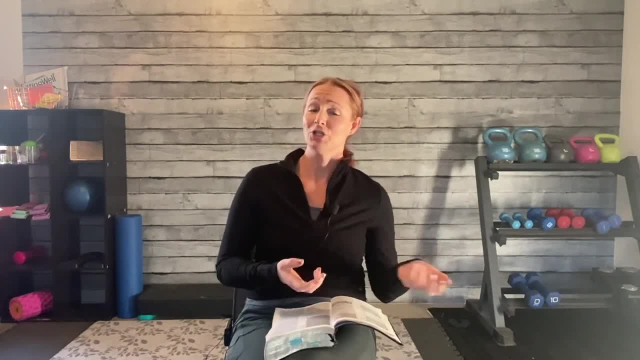 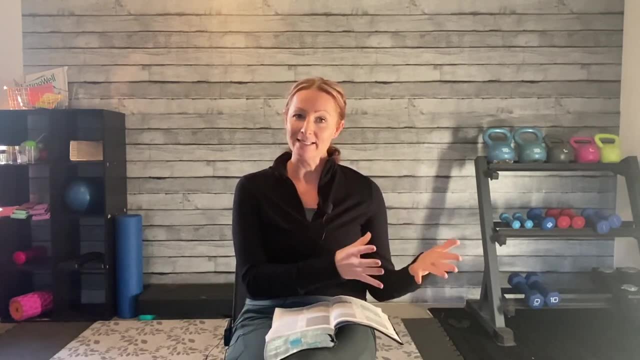 We're not going to put the wrong gas in, We're not going to pump it full of sugar and candy and then expect it to start running. It's going to have problems. It's not going to work because a car was designed to have a specific way that it's going to operate And our bodies are designed 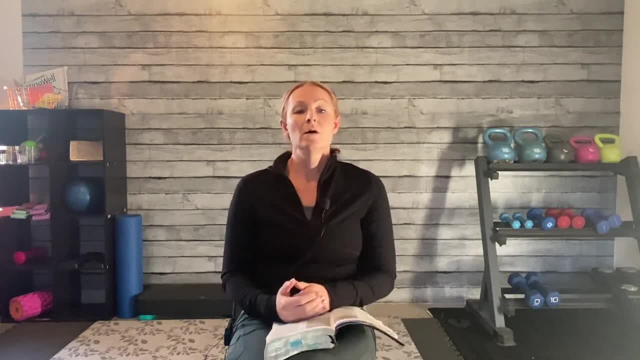 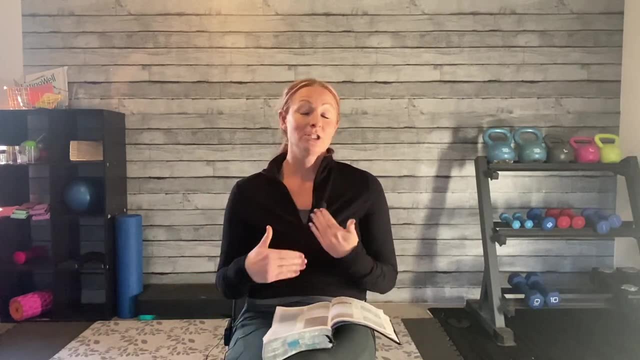 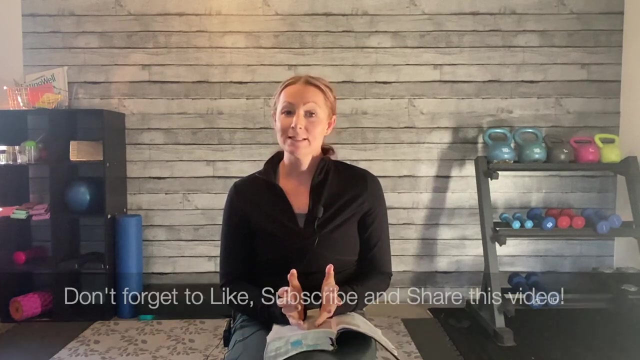 exactly the same, if not better. So God has created us. He's created the food for us, the herbs, the green food to nourish us, And that's what our bodies are meant to operate on. So I would just encourage you guys to try that And I really hope this is a blessing and maybe it.